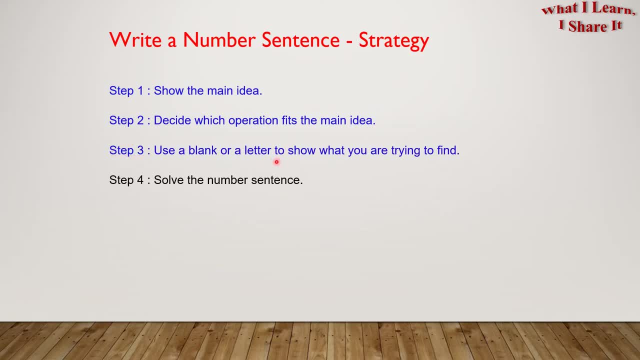 Step 3. Use a blank or a letter to show what you are trying to find. Step 4. Solve the number sentence. Here is a problem. to help us understand the strategy, Calvin has 15 shirts. Four of them were given to him by his mom and the rest by his dad. 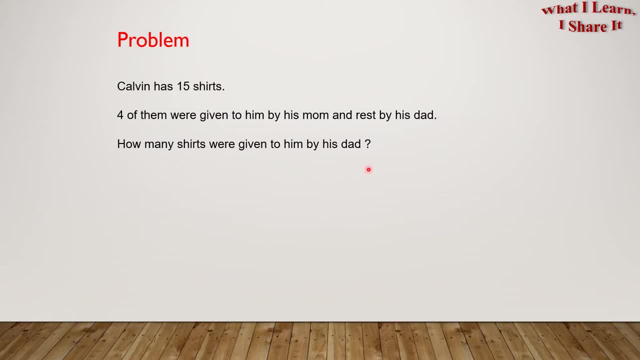 How many shirts were given to him by his dad? Do you want to try it yourself? Feel free to pause the video and try it yourself. Do you want to see how I solved it? I solved it in a step-by-step way. Let's see it. 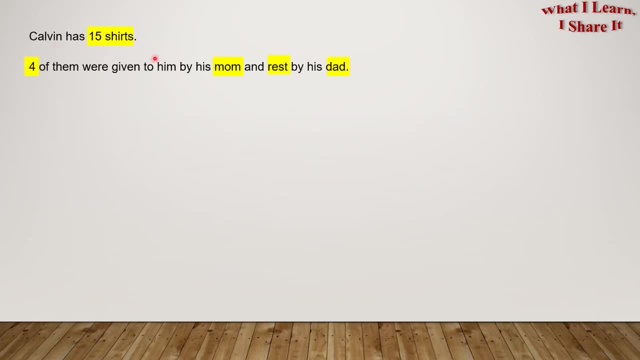 Calvin has 15.. Calvin has 15 shirts. 4 of them were given to him by his mom and the rest by his dad. How many shirts were given to him by his dad? Step 1. Show the main idea. So here in this pink block, we have all of Calvin's 15 shirts. 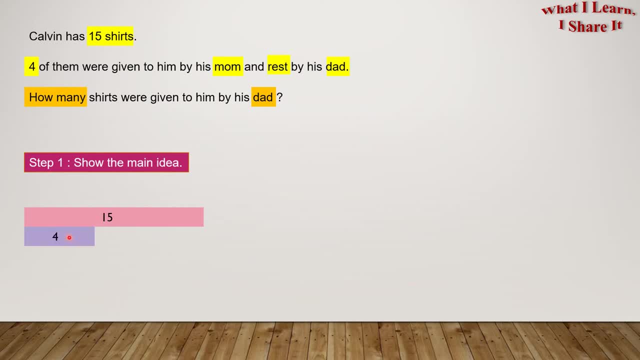 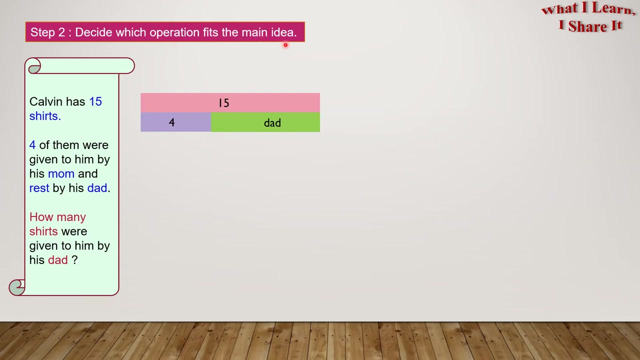 Then we know that 4 of them were given to him by his dad, his mom, and then the rest of them were given to him by his dad. step to decide which operation fits the main idea. so by operation I mean, like addition, subtracted, a subtraction, multiplication, division. so what will fit here to find: 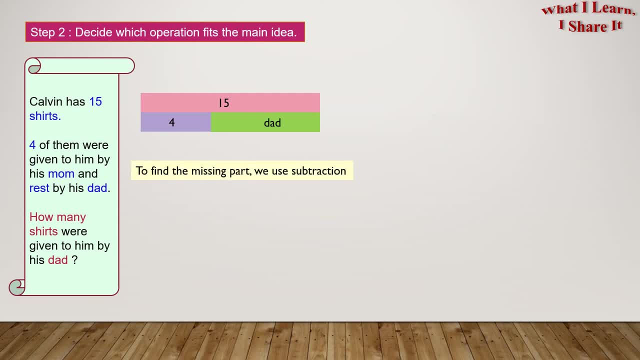 the missing part. we use subtraction. step 3: use a blank or a letter to show what you were trying to find. so here we are trying to find how many did dad give. step 4: solve the number sentence. so what will we do here? of course, we will subtract 4 from 15. here's how it looks like D equals 15.